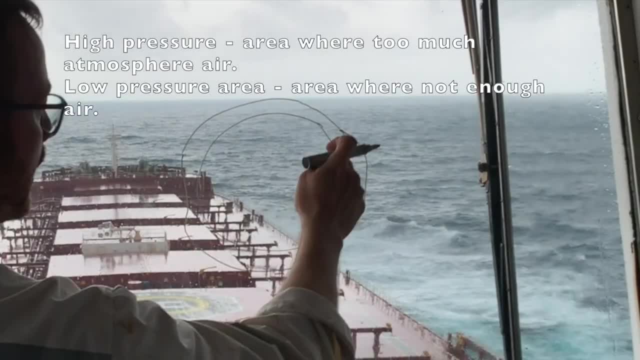 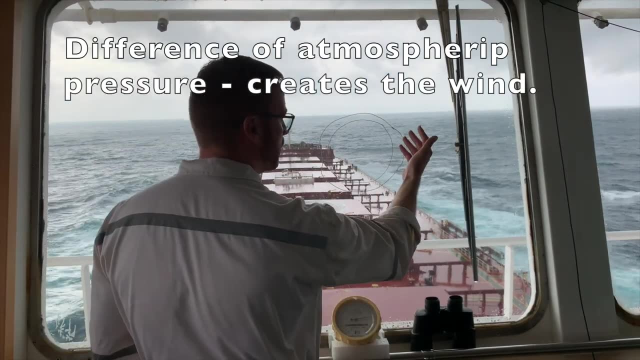 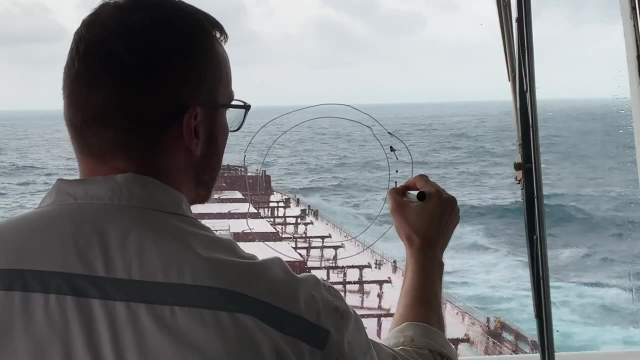 this area called low pressure area and this area is called high pressure area. Atmospheric pressure creates the winds. The high pressure is the pressing the mass of the air on the sides from its center. The air is pressed away from the center of the high pressure. On the low pressure we have. 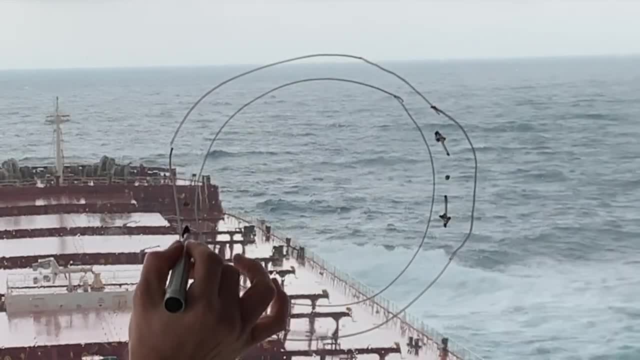 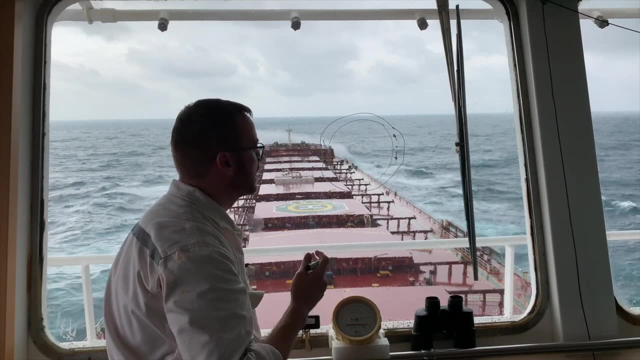 something opposite. The air mass is trying to compensate the low pressure. That's why the air is going to the center of low pressure. From this aspect, it's difficult to understand how the wind is blowing, but if we see from the top, like we are doing this from the space, 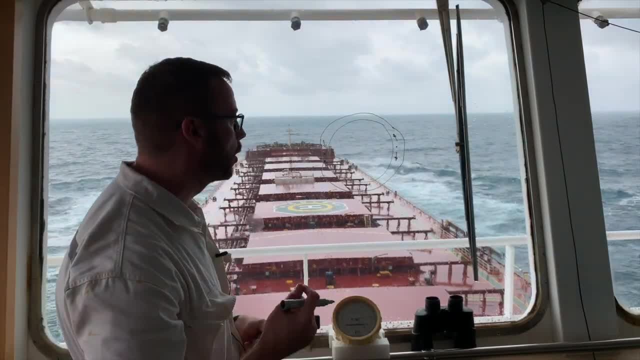 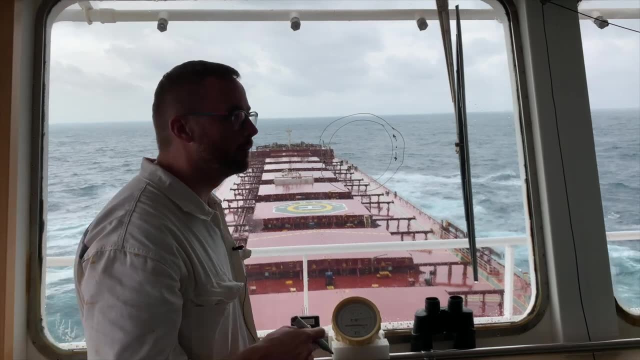 we will understand how knowledge and understanding of the low pressure area and high pressure help us to understand what is going on in the area we are sailing. First of all, in northern semicircle and south semicircle, the low pressure and high pressure behaves. 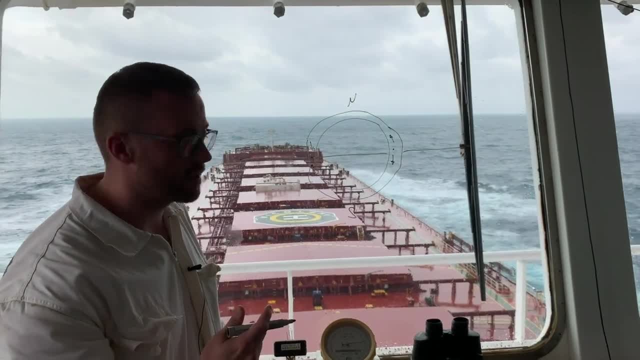 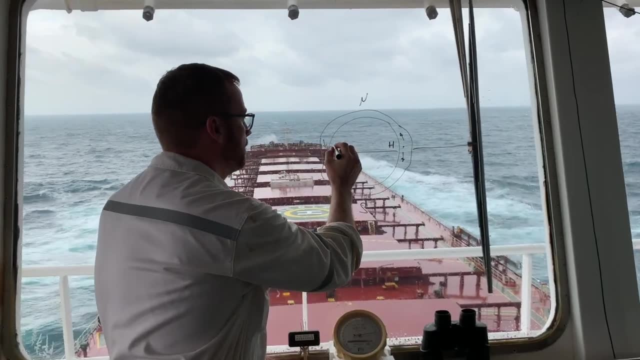 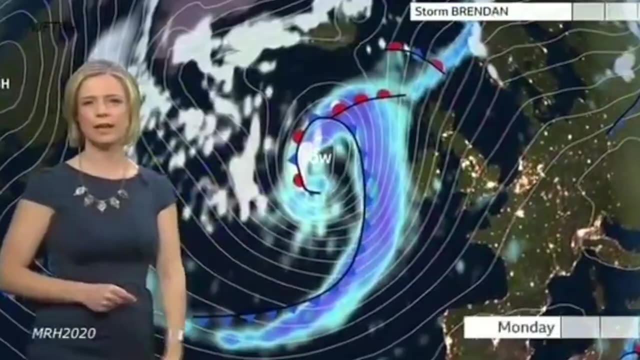 different. In weather charts and in forecasts the high pressure is marked as H hotel, The low pressure marked with Lima. Lima means low, H hotel means high, Further south. Now, Monday's weather is going to be dominated by Storm Brendan, this deep. 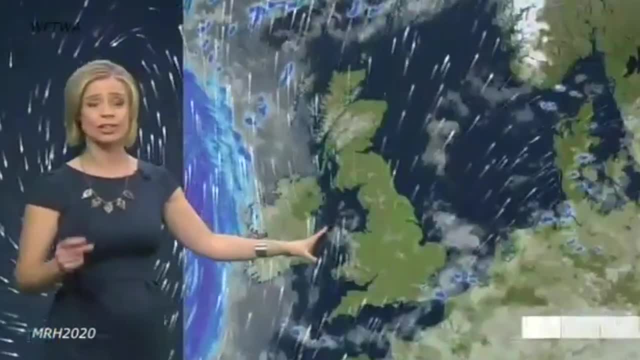 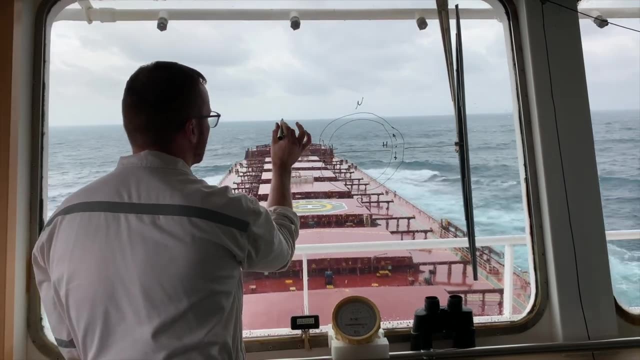 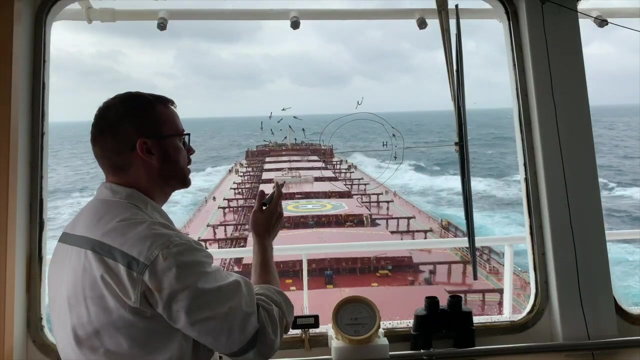 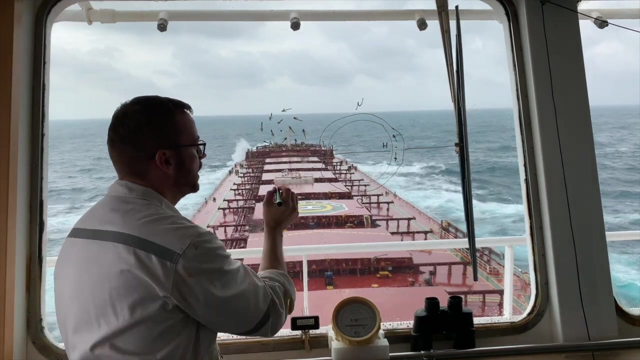 area of low pressure moving its way in from the Atlantic on a strong jet stream In the northern part of our planet, above the equator. the low pressure In northern semicircle, The low pressure, Always has anti-clockwise direction of rotation. In the south semicircle we have something opposite. This is the nature of our planet, and I don't know exactly how does it work, but above the equator, low pressure always goes anti-clockwise. Below the equator, low pressure always goes clockwise. Actually, when you are flushing the toilet, you are not flushing the toilet, You are flushing. 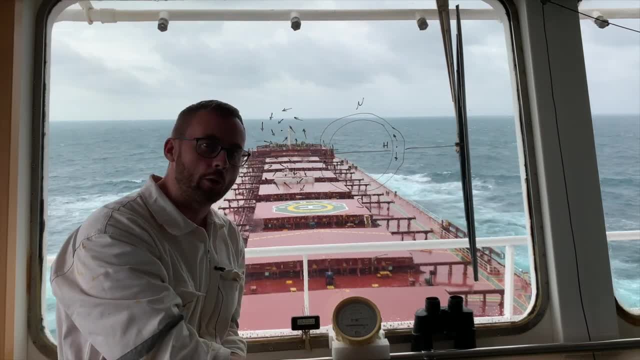 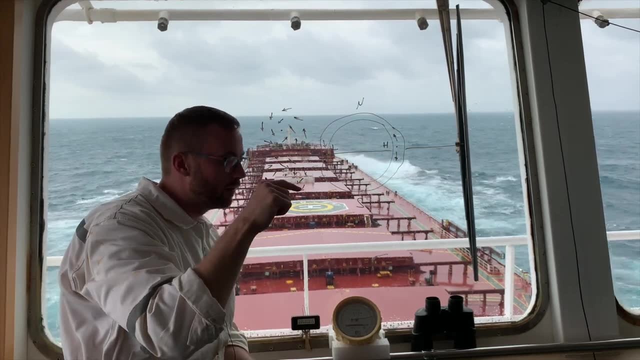 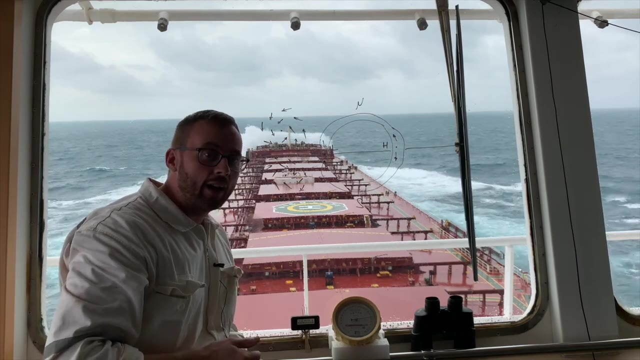 the toilet, You are creating the low pressure in your toilet bowl and it will work exactly like this. If you are somewhere in Europe, you will flush the toilet and the water will rotate anti-clockwise. If you are in Australia and you will flush the toilet, the water will go clockwise. 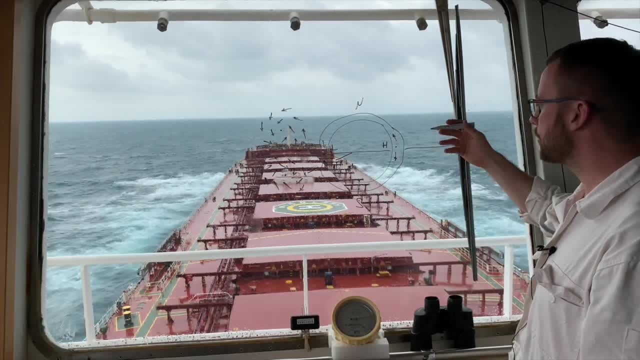 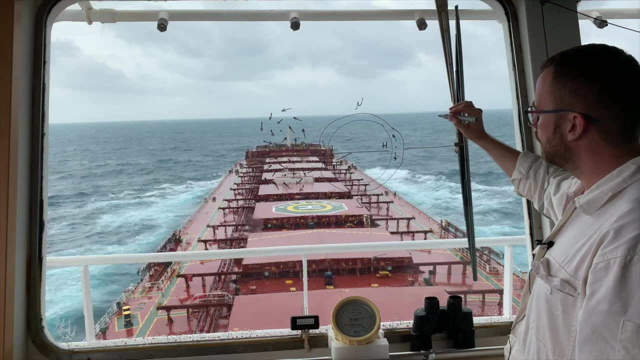 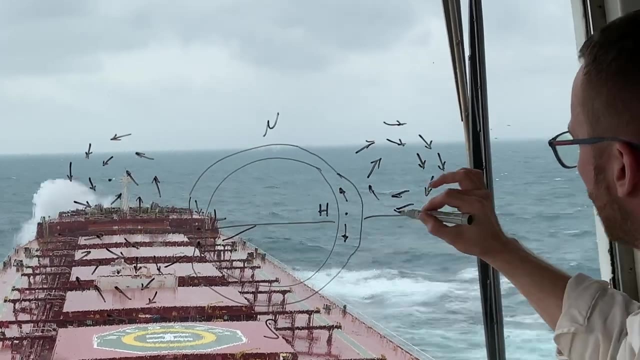 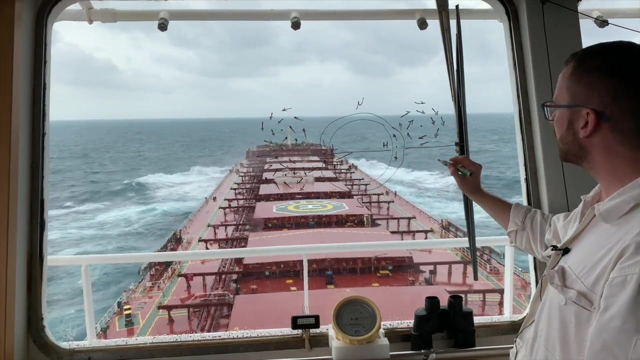 If we talk about the high pressure, the behavior of high pressure area in the above the equator and below the equator also different. Above the equator the high pressure is rotating clockwise and, respectively, in below the equator it's rotating anti-clockwise and actually for the moment we have a 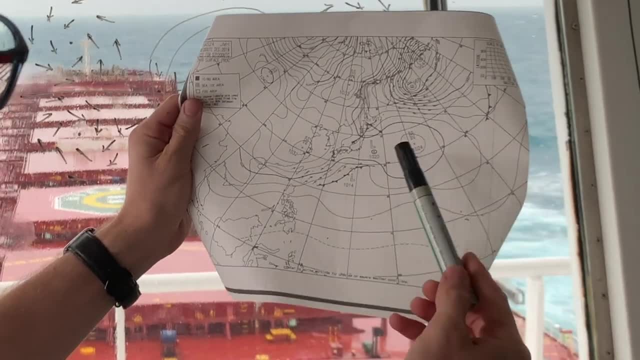 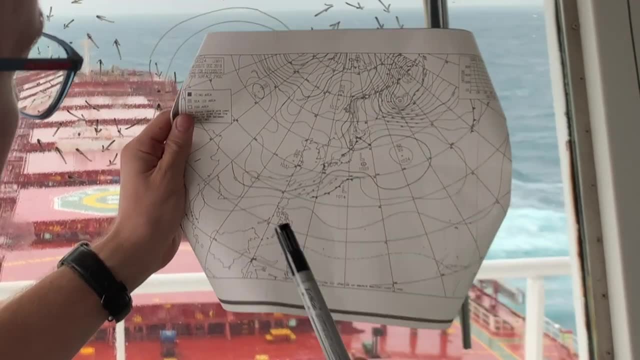 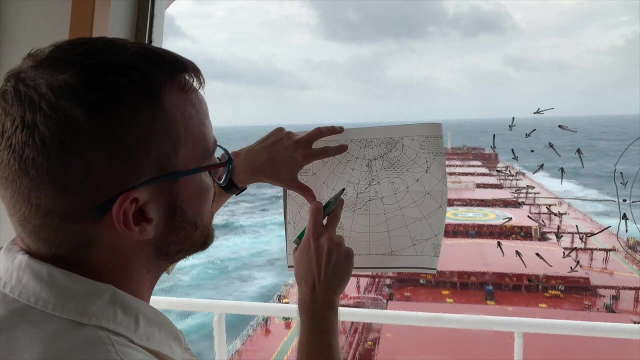 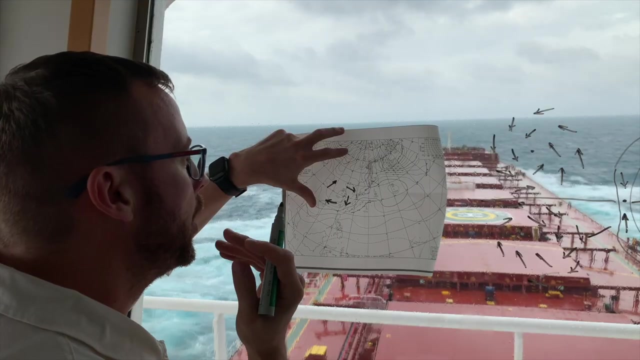 weather facts chart where we can see the distribution of high and low pressure areas among the area of the globe, and we can see here high pressure, high pressure, low pressure 964, low pressure 968. in this area atmospheric pressure is very high, so wind will blow clockwise from the center, knowing that in northern part 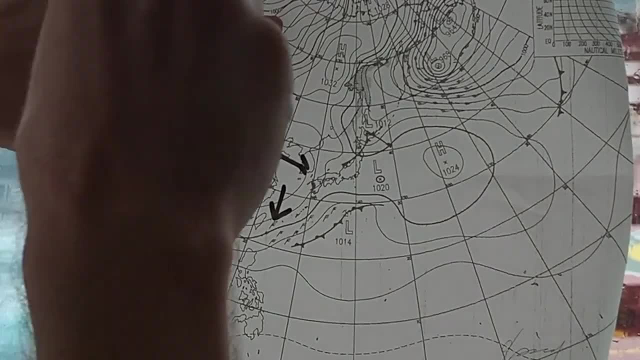 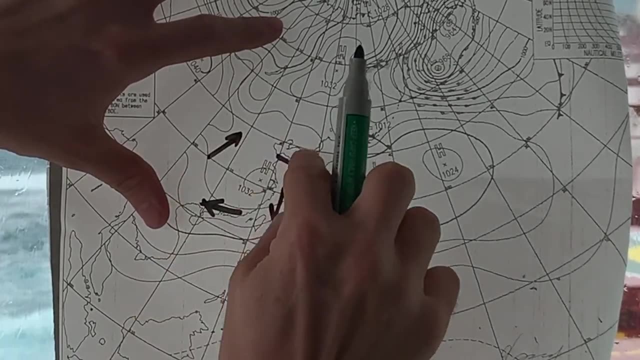 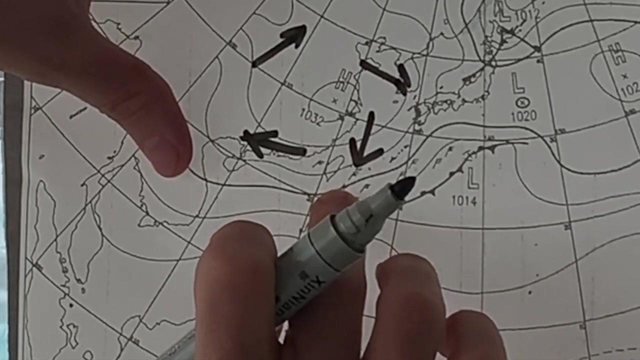 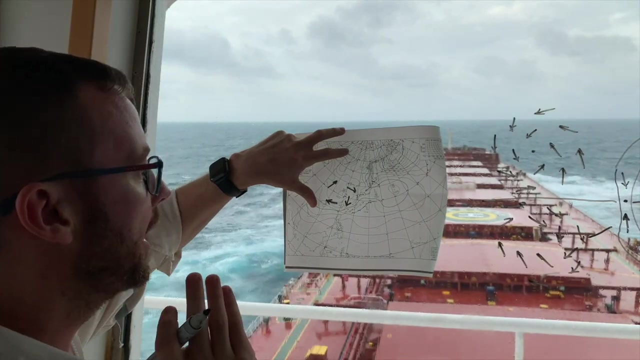 of our planet. the air is circulating clockwise around the high pressure. the winds will go clockwise. as you can see, these small arrows are giving us the warning. be careful. there are strong winds over 30 knots and it is completely according to the things I've been talking on this sketch. here is the low pressure area in. 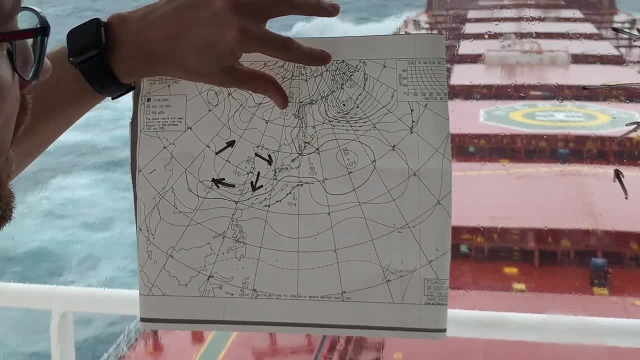 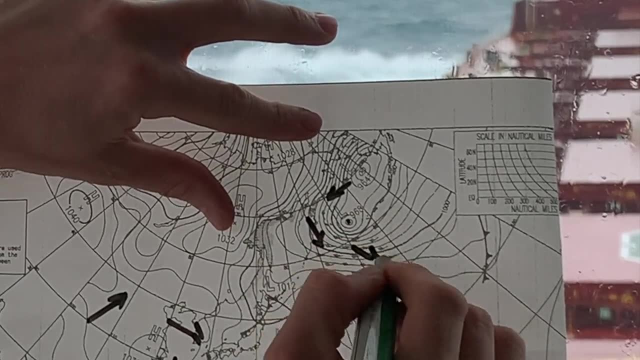 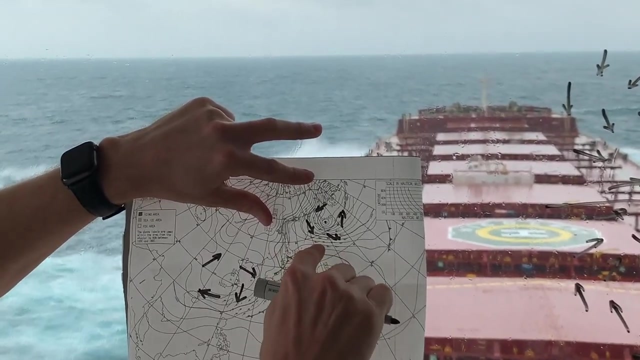 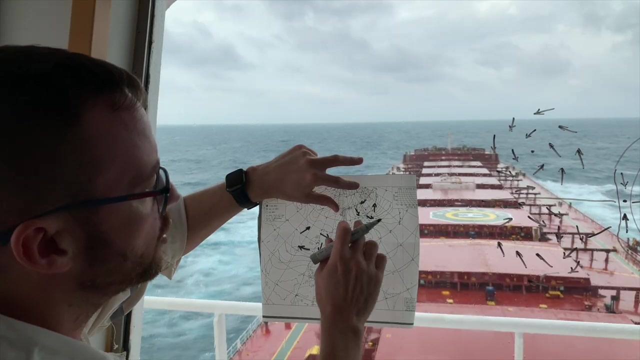 the northern part of our planet, the air is circulating anti-clockwise around the low pressure area and, according to this chart, we are absolutely right, because we see that weather chart is giving us the warning: be careful, the winds here are over, then not sometimes to low pressures can merge together and we will have more stronger. 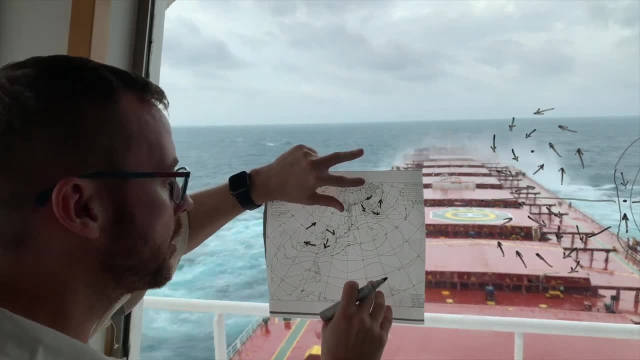 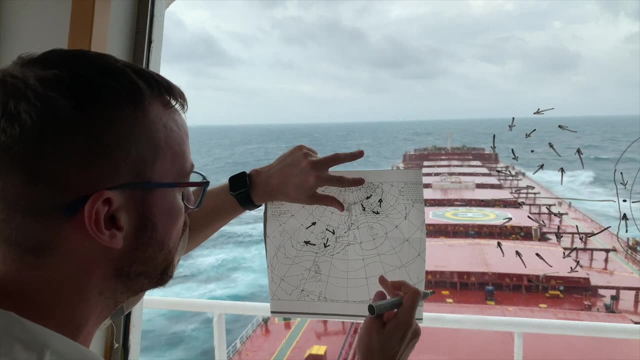 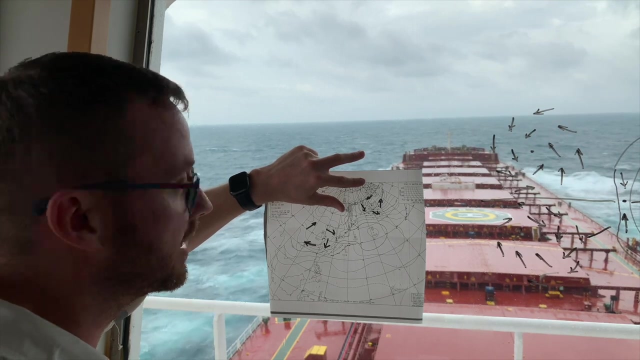 low-pressure area. extremely strong low-pressure areas which are forming in this part of the globe, near the philippines, in Pacific Ocean and moving here in the direction of China and Japan, is called tropical storms, the typhoons. and now the question: what advantages is giving to us?